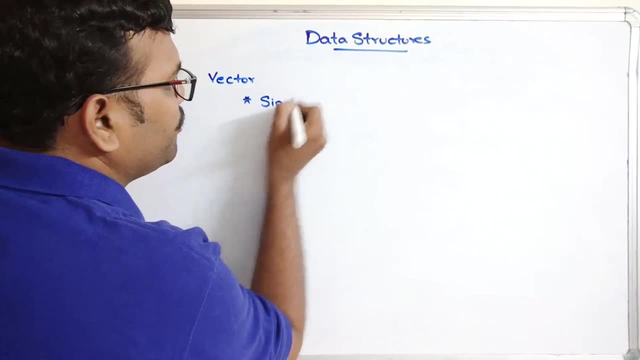 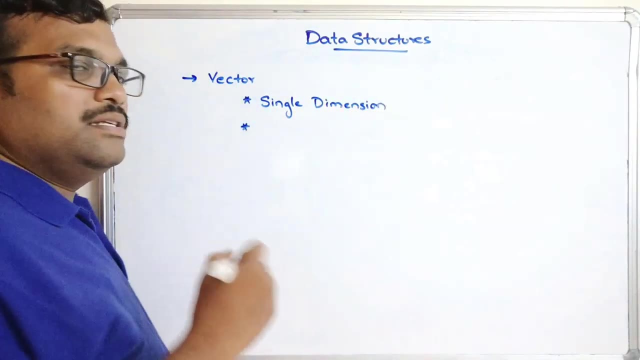 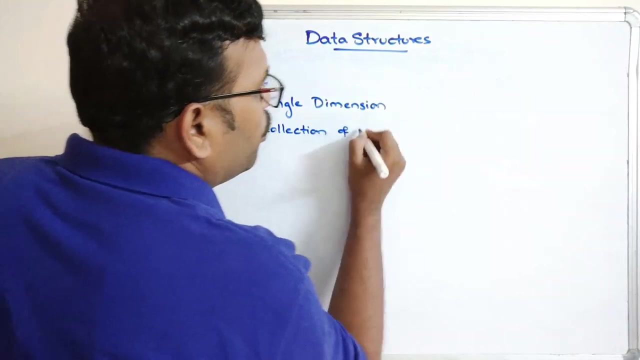 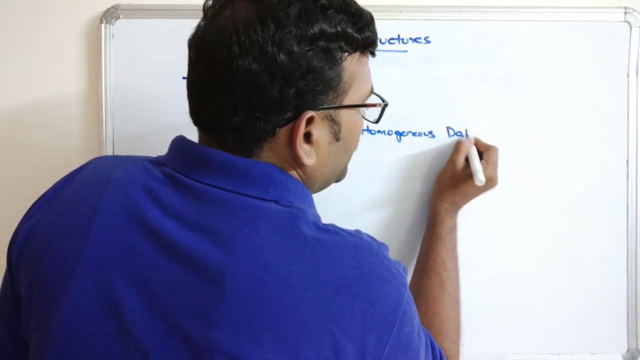 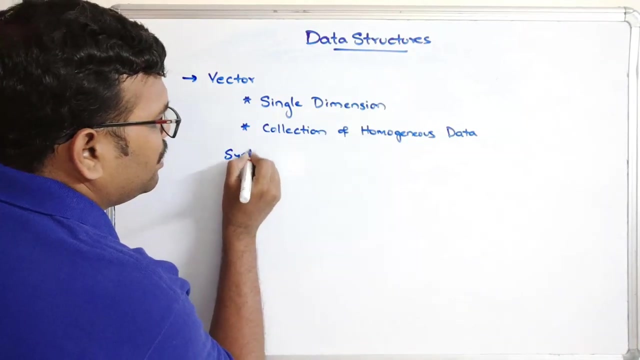 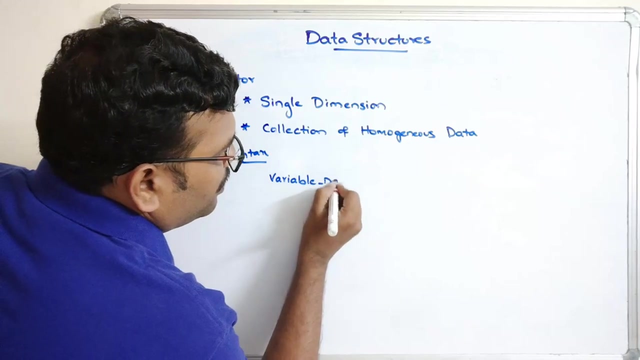 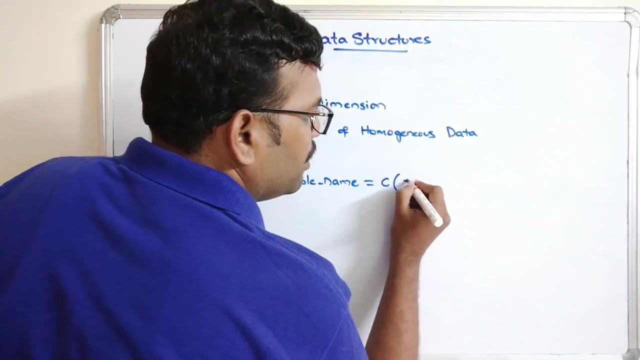 this is a single dimension and this is a homogeneous data. It's a collection of homogeneous data. That means it will be having the elements of same data type And the syntax for vector is some variable name, or we can say it as: a vector name is equal to C of element 1,. 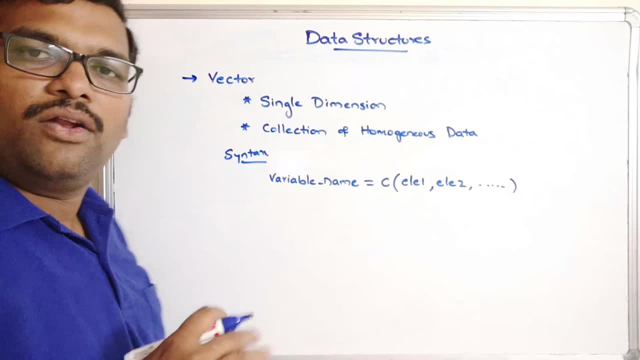 element 2,, element 3, element 4,, element 5,, element 6,, element 7,, element 8,, element 9, and so on. So here all the elements should be of same data type. So either it can be. 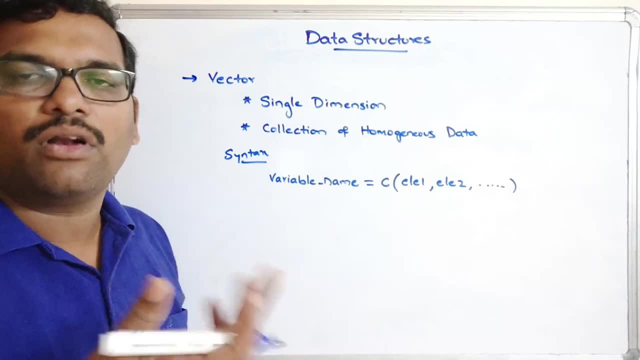 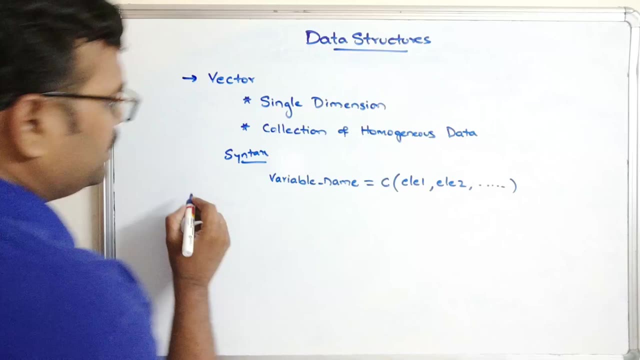 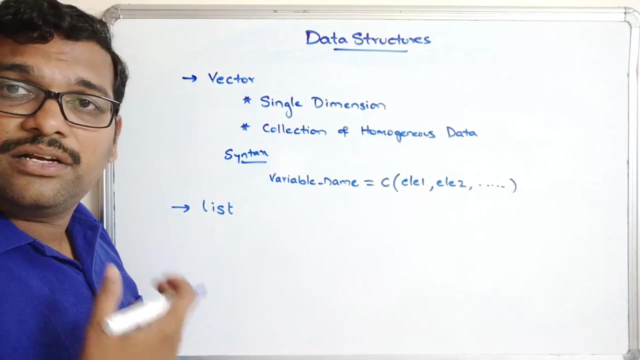 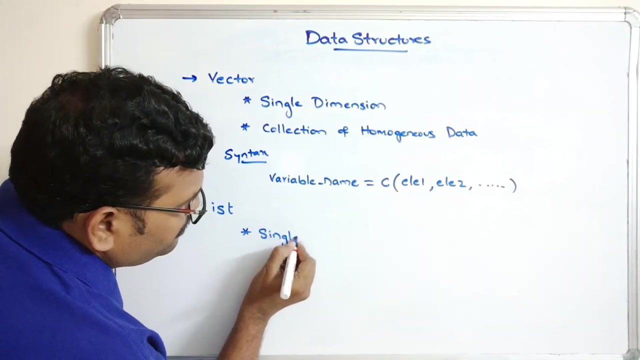 integer, or it can be a float, or it can be a string or character data types. So this is syntax for creating the vector data structure And the second one is a list. So list data structure is also similar to the vector. This is also a single dimension. It's also a single dimension, But it is nothing but. 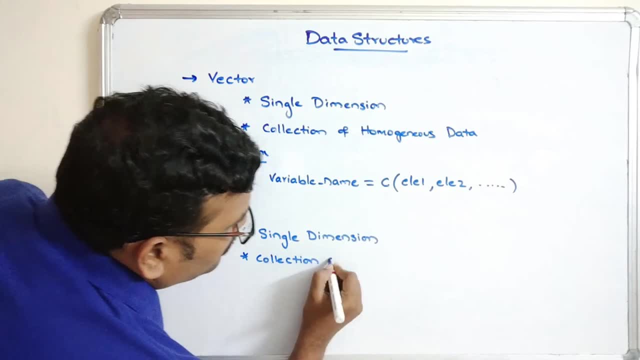 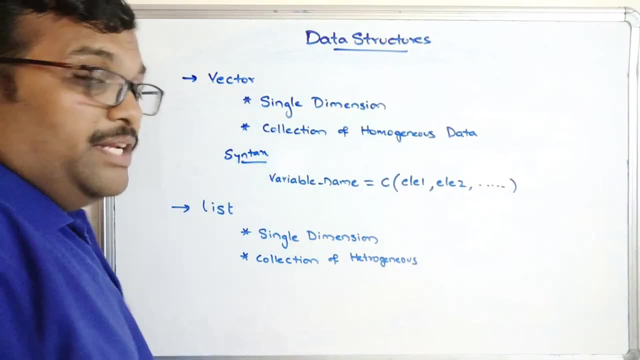 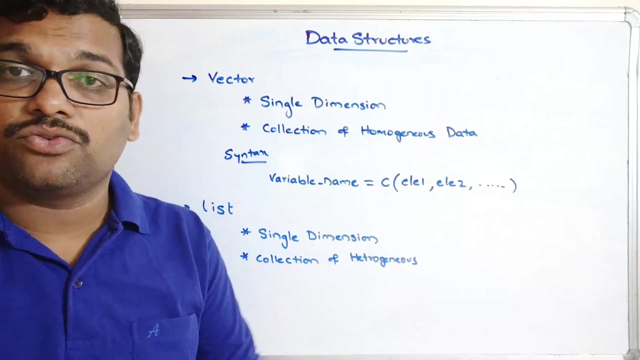 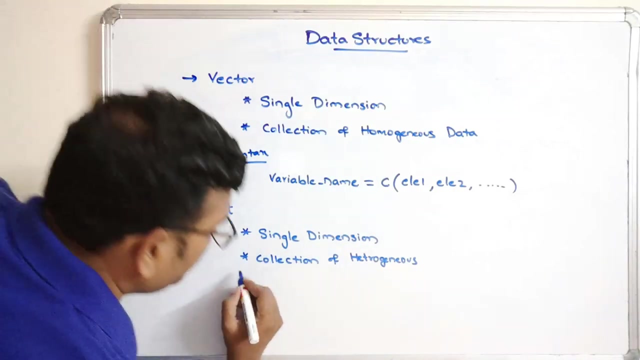 a collection of heterogeneous. Collection of heterogeneous, That means it is a collection of elements, multiple elements of different data types, So we can store all the elements of different elements. So that's a main difference over list and vector And here the syntax for creating a 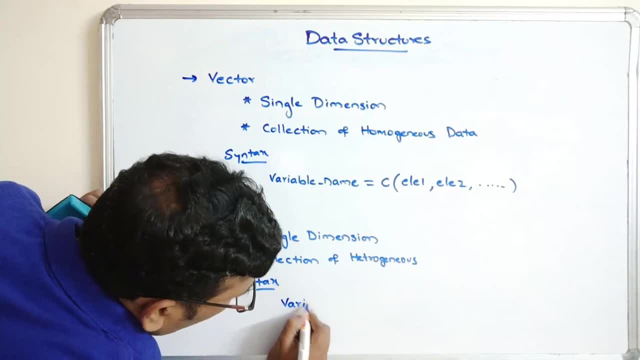 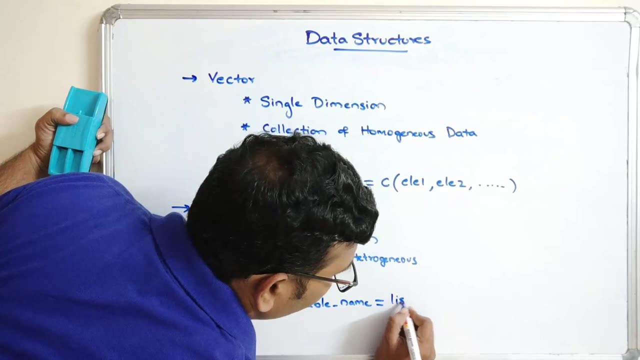 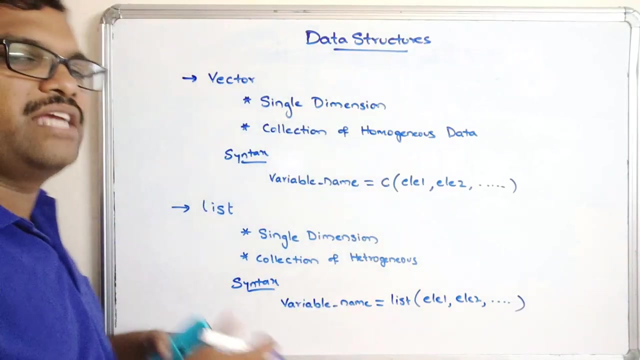 list is a variable name, or we can call it as the list name. Variable name or list name is equal to user list function, followed by element 1,, element 2, and so on. So here the elements can be of different data types. So here elements should be of same value. So 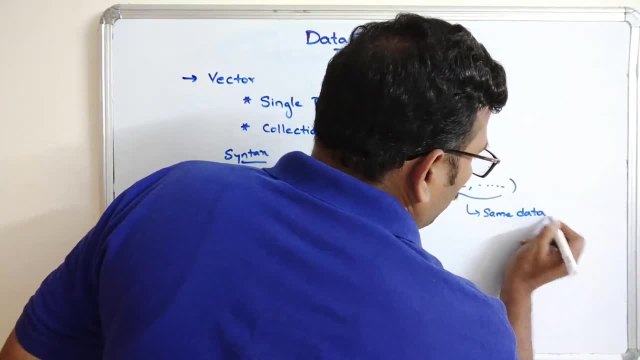 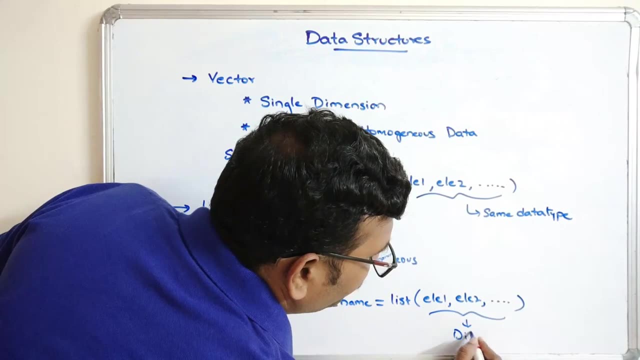 all the data types in a text box, Unless. if you have questions regarding graphics, Then data type, right. that that's why we are. we are calling it as a homogeneous data and here it can be of different data type, different, so no need to worry about. 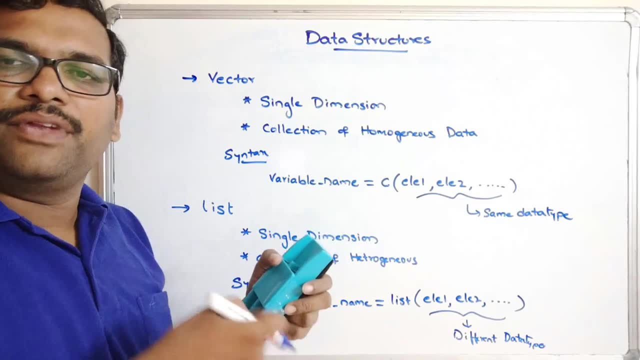 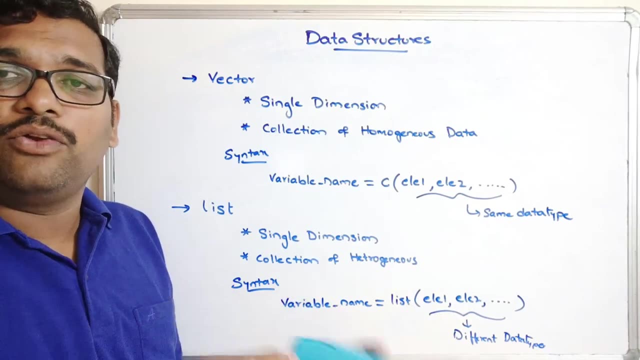 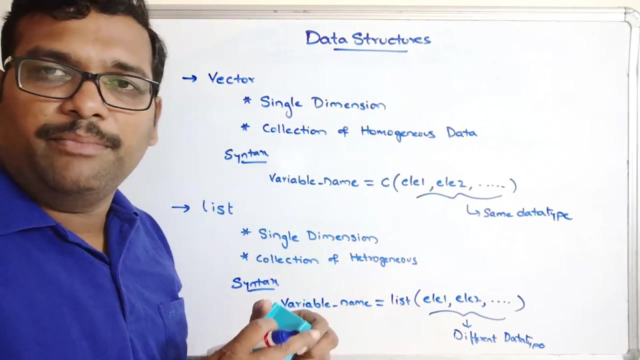 all these things. I implement each and everything in the R studio. so we'll execute a small program, just, will create a vector and will print the vector, will create a list and we print the list. okay, for all the data structures. I will show you the implementation. so don't worry about this. so just we'll see the. 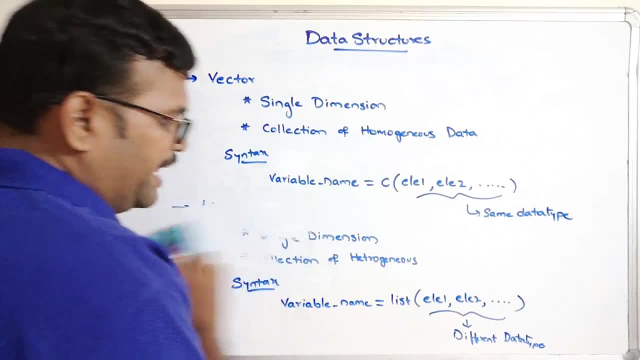 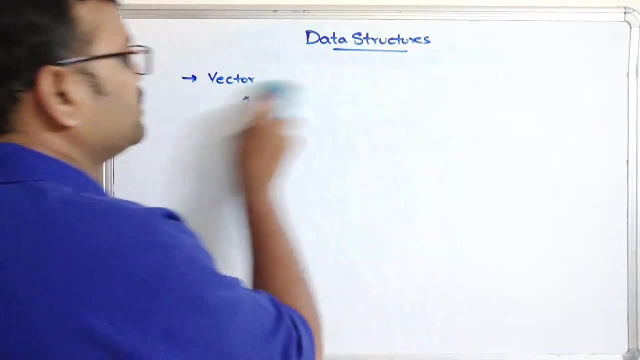 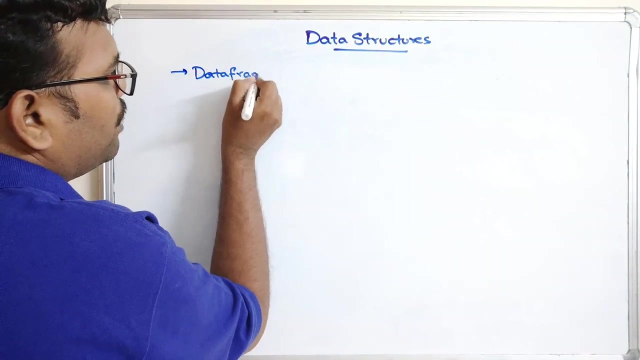 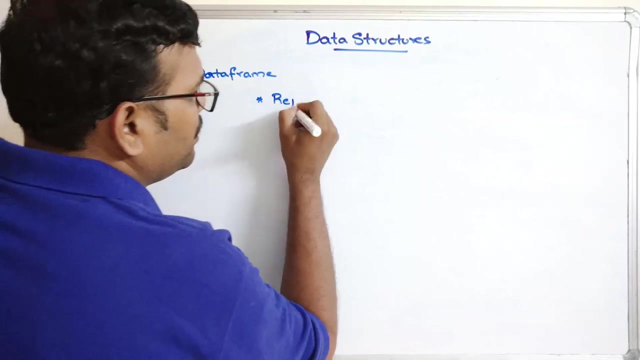 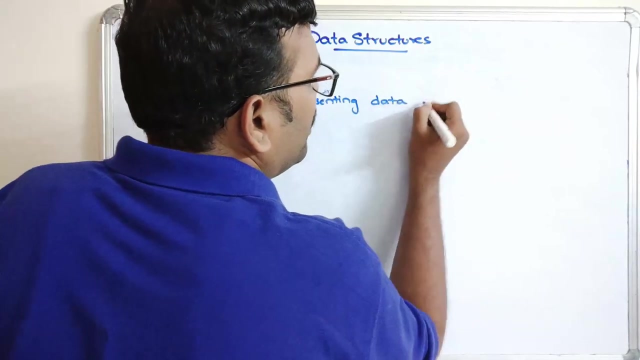 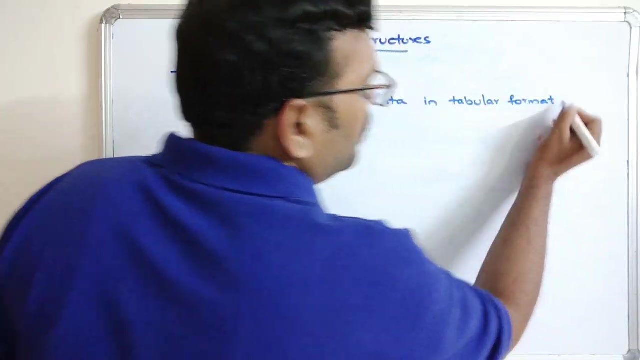 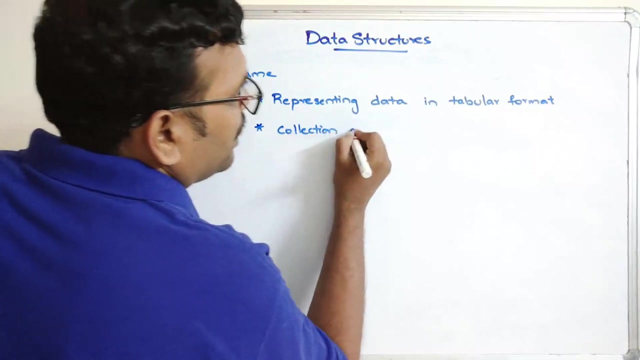 syntax part. now the two things completed. then, third, data structure is a data frame. third, data structure is a data frame, so a data frame is a tabular data, representing data in tabular format. so it forms a table right, so it can be a collection of vectors, collection of vectors, collection of. 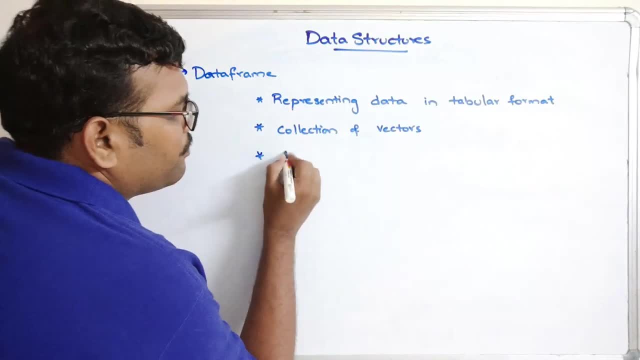 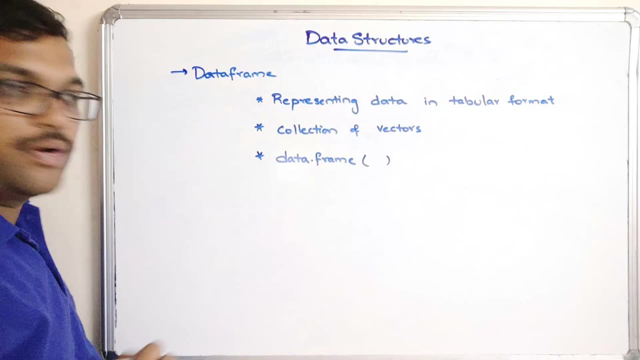 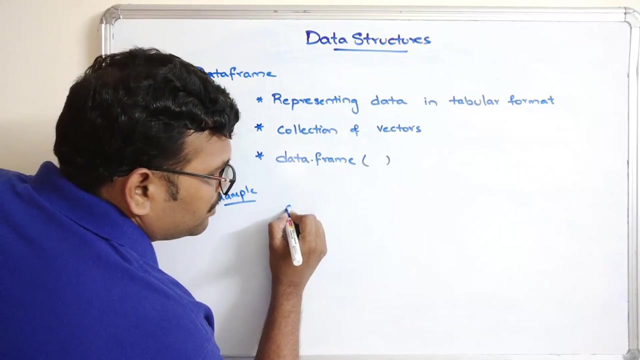 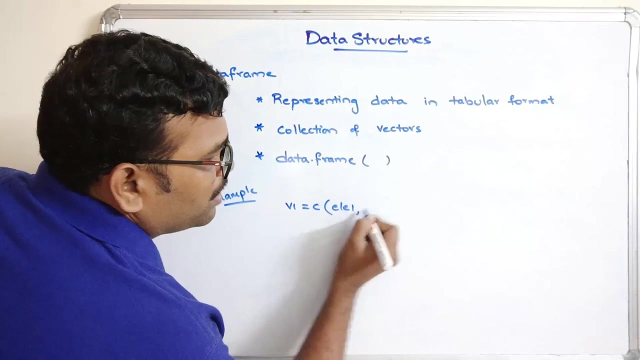 vectors. so for this we have to use the function called DATAFRAME function. DATAFRAME function, right, so example here I will give an example. let us take some vector 1- see v1 is equal to C- of some element 1, element 2 and so on. and vector 2. 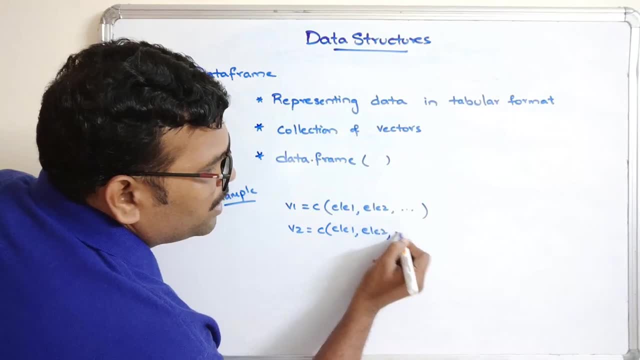 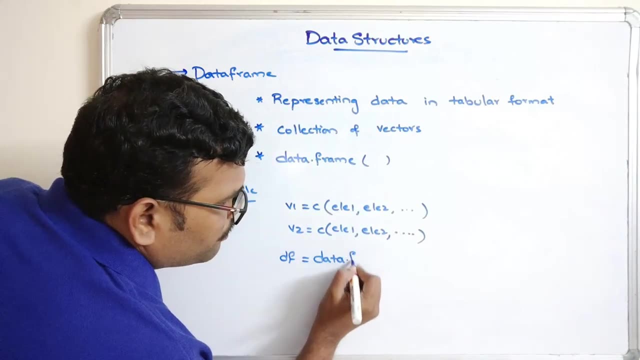 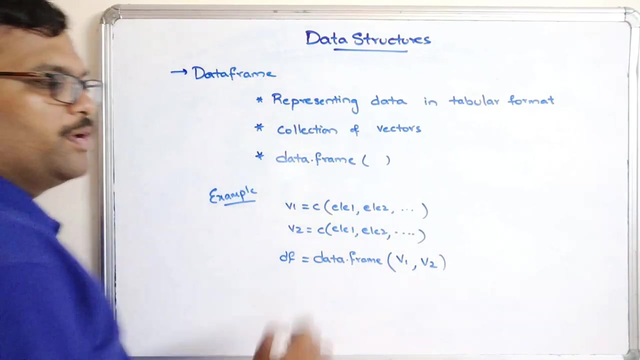 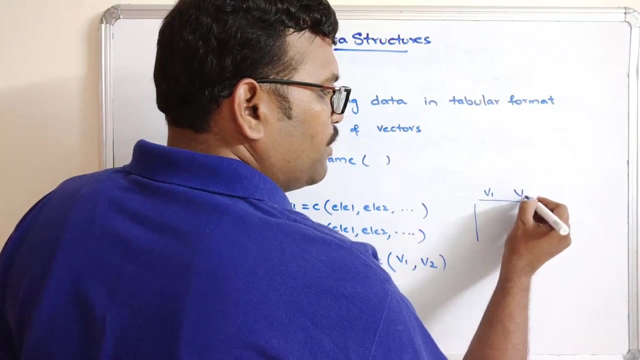 of element 1, element 2 and so on. and now you can go with the data frame is equal to data dot frame function and pass on these vectors: v1, comma, v2. so obviously, if you execute the program, you will get the data in a tabular format, like giving a names as v1, v2 and indexes as 1, 2. 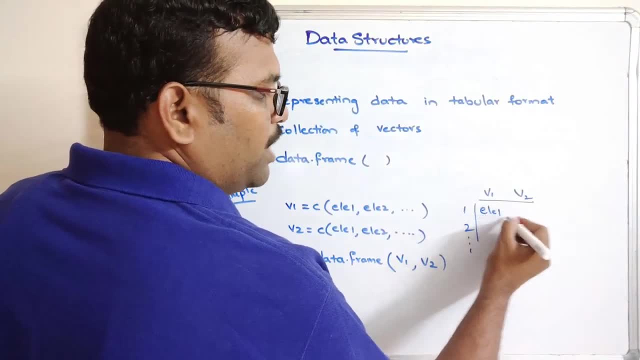 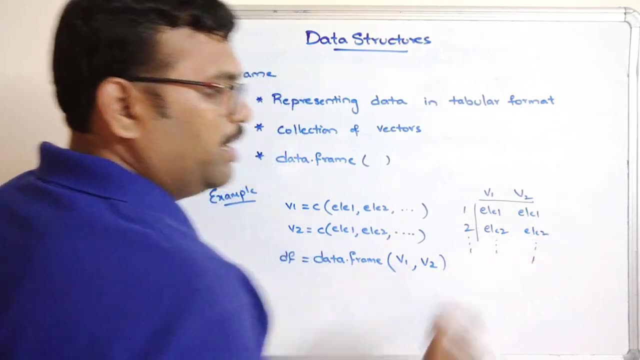 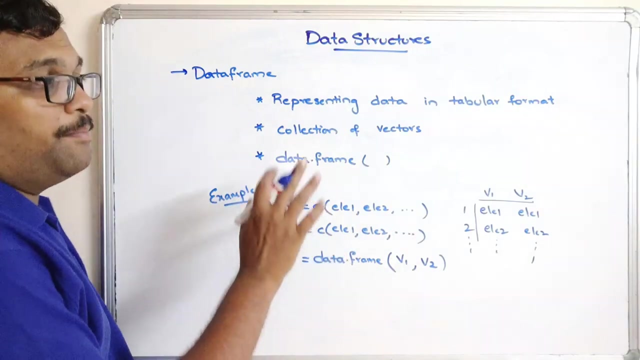 and so on. so you get an element 1 and element 2 and so on, and here also we'll get element 1, element 2 and so on, right? so in this format that output will be displayed. that means it will represent the complete data in a tabular format. so that is the data frame. data structure, data frame. 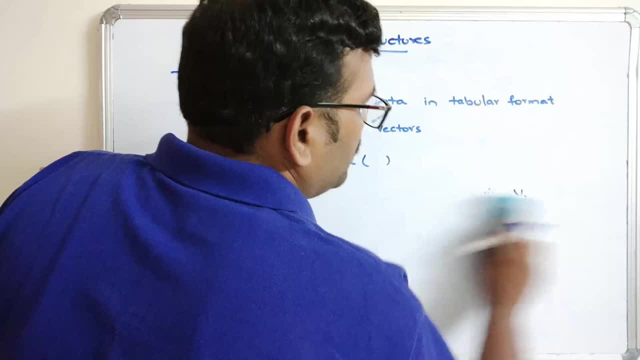 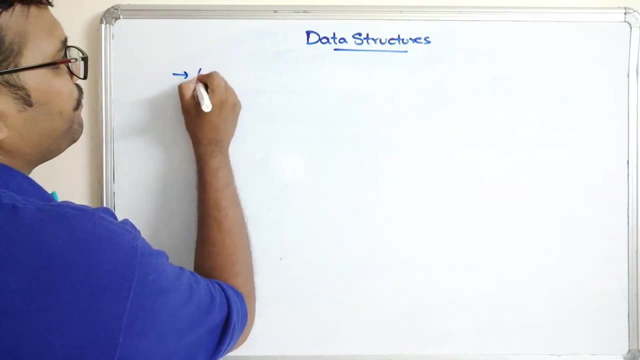 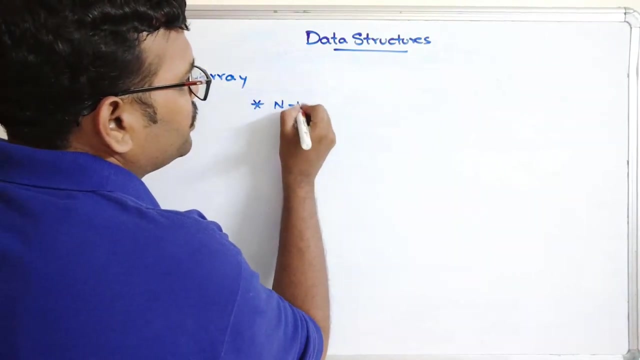 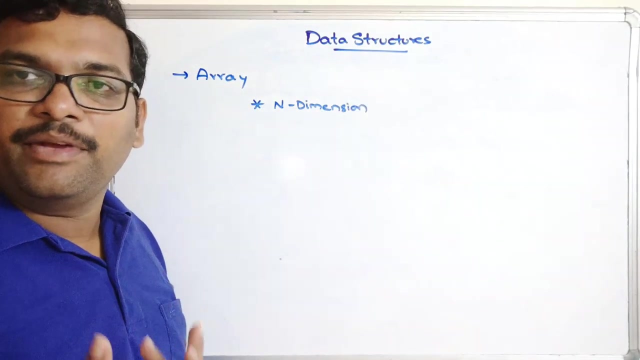 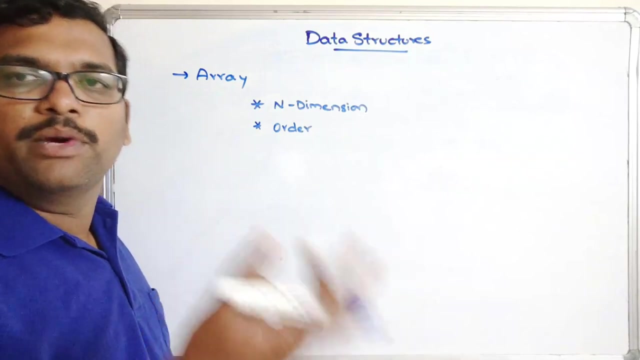 then the next one. so is an array. so array is a n-dimensional representation. we can represent the data in a n-dimension, n-dimension, and here we'll give some order order of data. let it be some: 2 by 2, 2 by 3, 3 by 2. 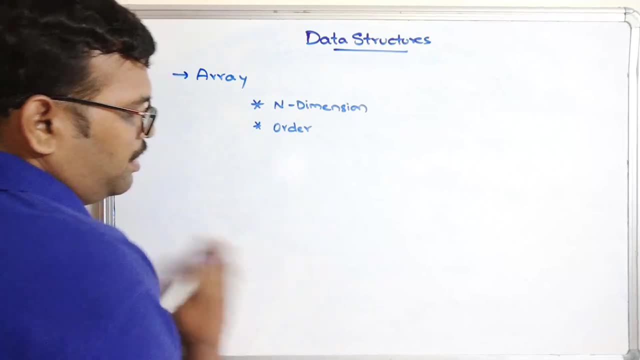 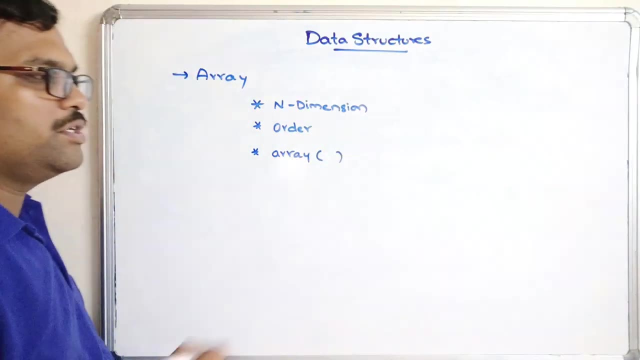 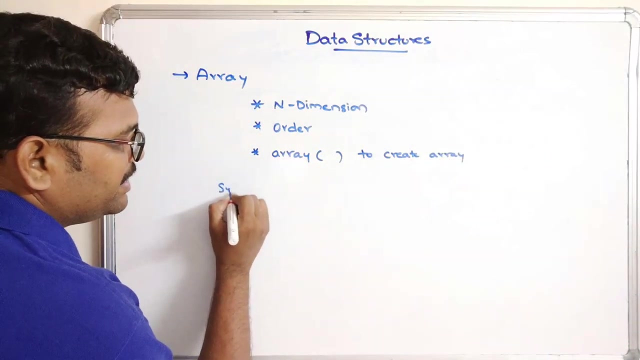 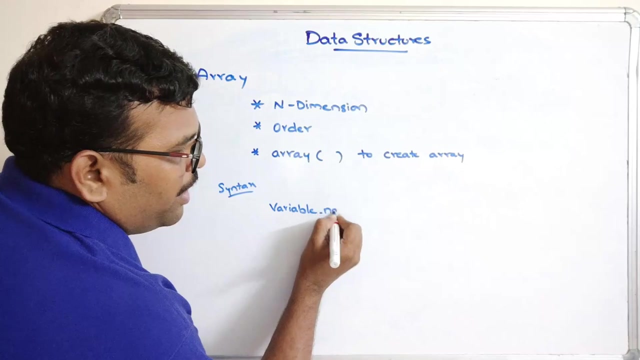 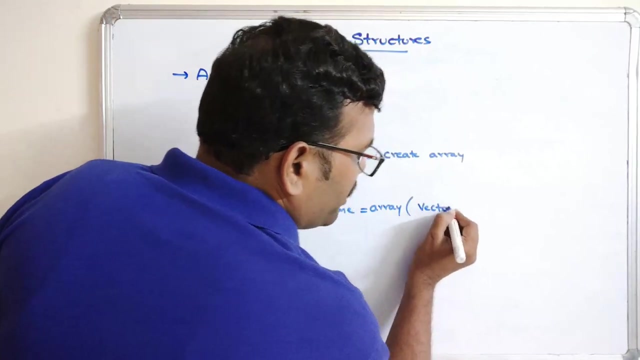 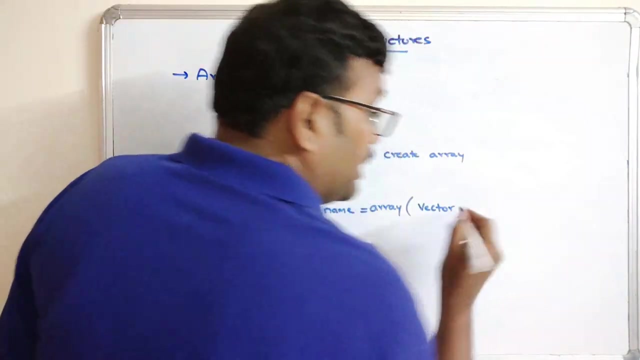 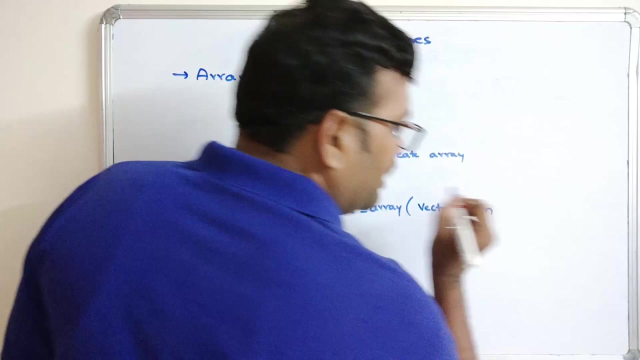 right, like that. so here, so It will accept. I mean we have to use an array function to create an array, Array function to create an array, Right, And the syntax for this array is some variable name or array name. Okay, Give the variable name or array name, Give the array, Give the vector here The complete vector, Complete vector, And the second parameter will be the dimension. So the dimension should also be given as a vector In terms of vector, Right? So for that I have to give that DIM parameter A parameter name called as a DIM, Which is called as a dimension. 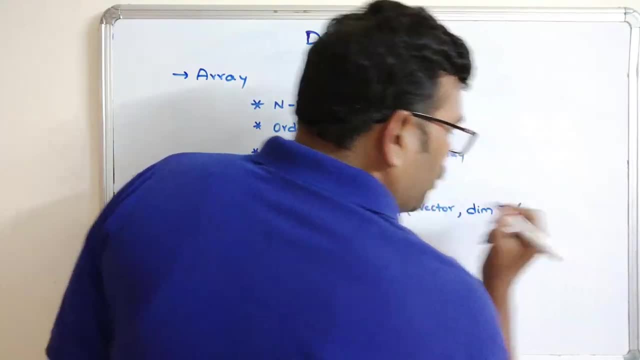 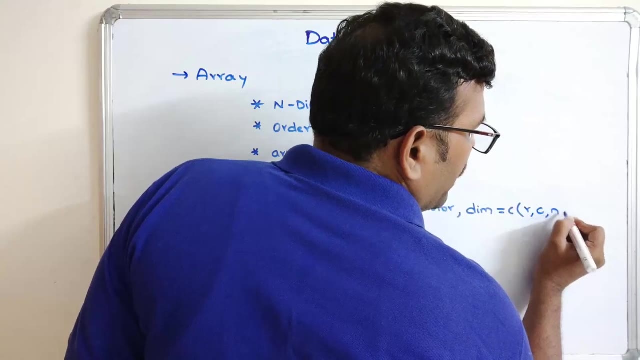 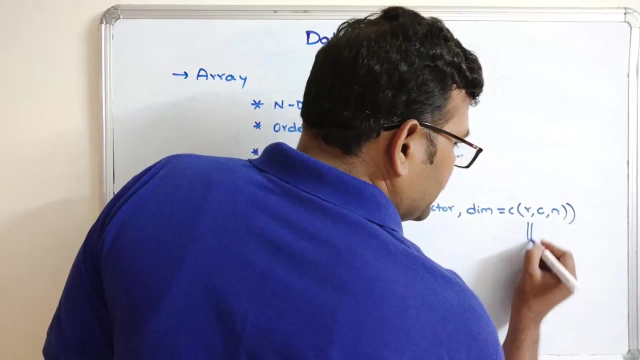 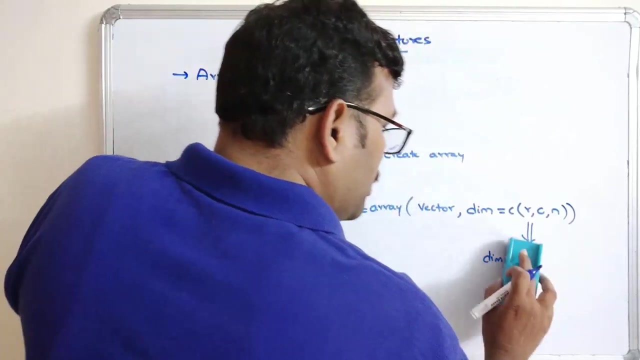 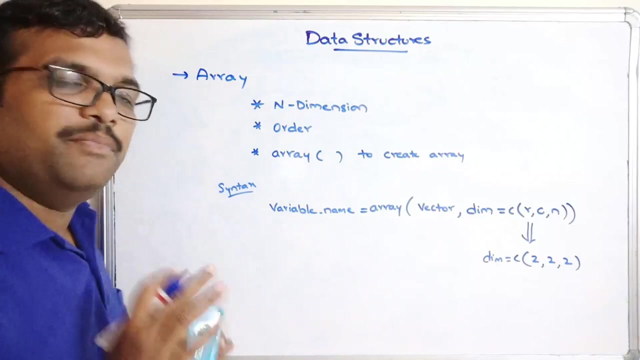 So dimension is equal to, to vector. so it consists of three things. one is rows, columns and number of arrays: rows, columns and number of arrays. so if this dimension, if this dimension is C of 2 comma, 2 comma 2, that implies that means whatever the vector here we are giving. so 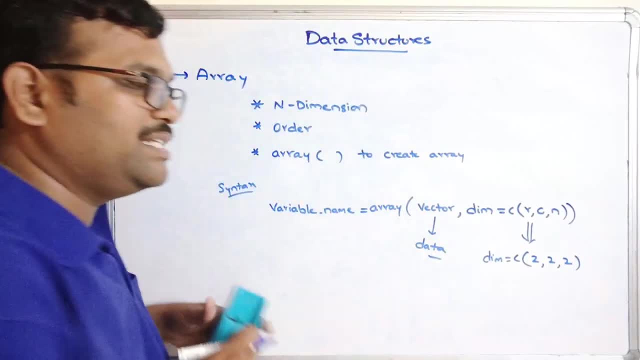 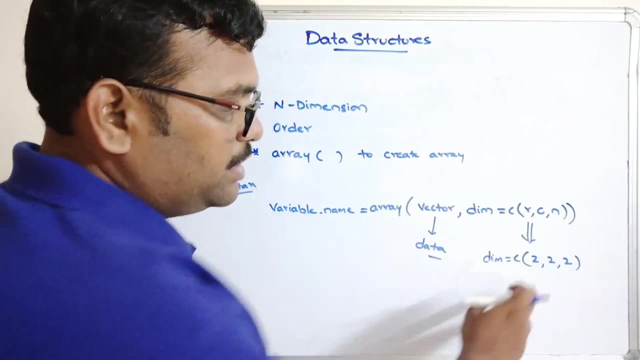 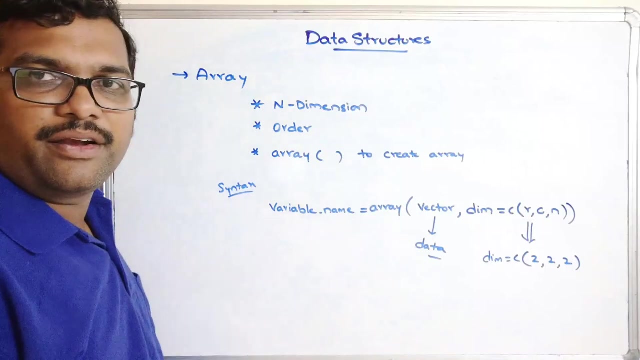 this is completely data. the vector is a data right, so this data will be arranged in a 2 by 2 array of two arrays. so this is a rows columns and this is a number of arrays, right. so 2 arrays with the order 2 by 2 will be created, and if you are giving here 3, that implies 3. 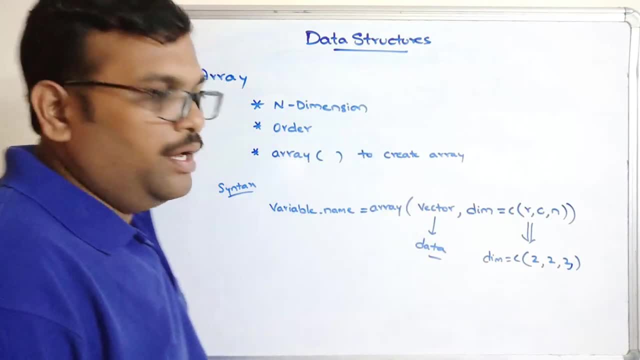 arrays with the order of 2 by 2. that implies 2 by 2. so here now, if we were to see it as an array, arrays with the order 2 by 2 will be created right. So the first one row, column and number. 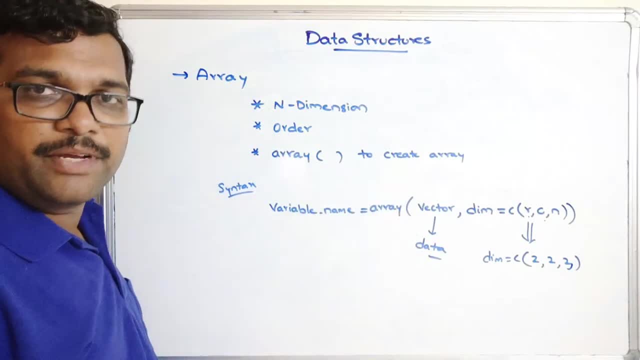 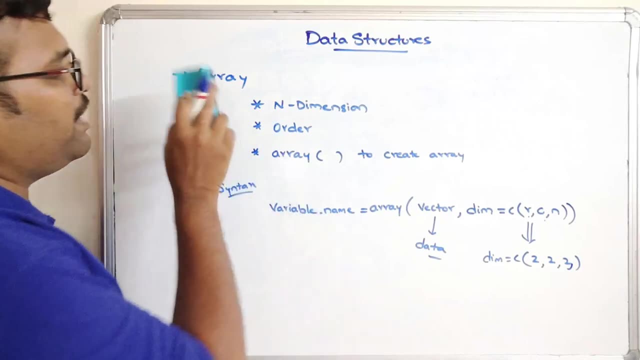 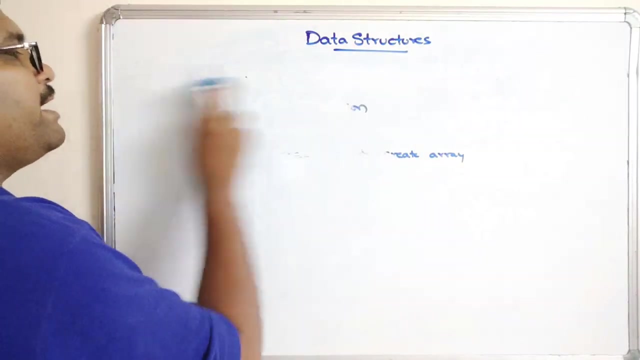 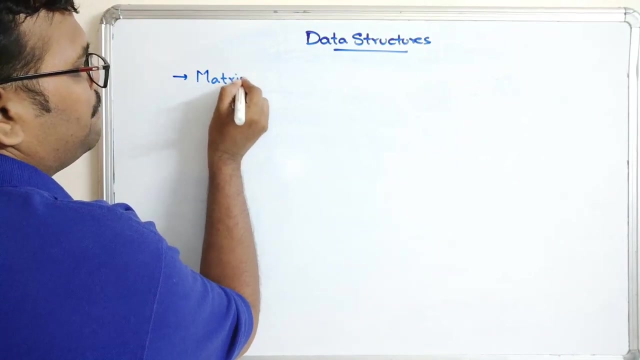 of arrays with particular dimension, with a particular dimension, right. So these two are the parameters we need to give for array function in order to create an array. And the next one, and the last one, is a matrix- matrix, See matrix. So matrix also will. 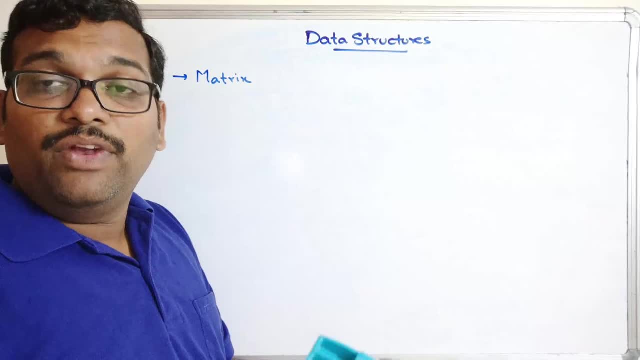 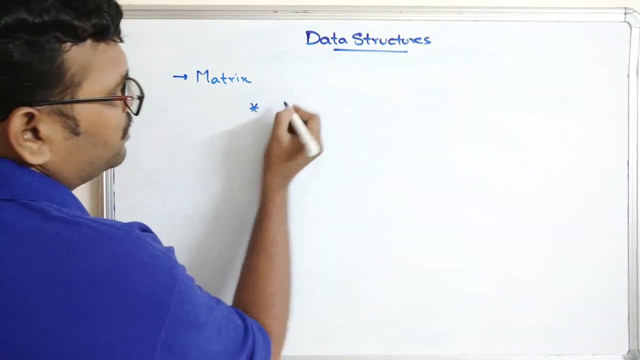 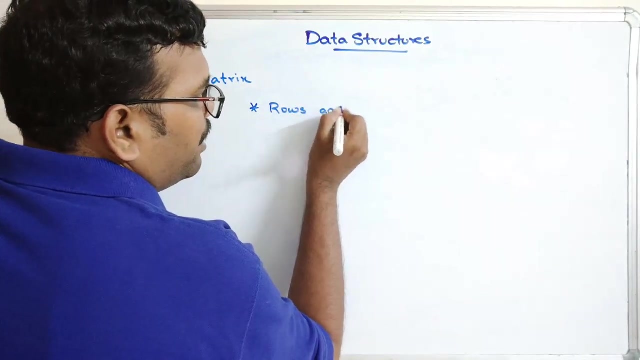 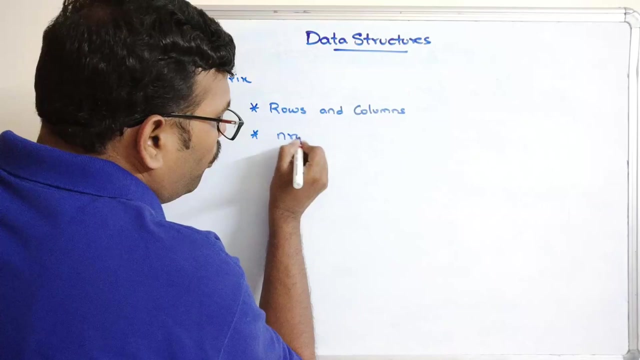 create in terms of rows and columns, right. So we will represent a matrix order as a rows: number of rows into number of columns. So here also the same thing. So this is also rows and columns. the data Data will be represented in rows and columns, right. So here we need to give the n row. 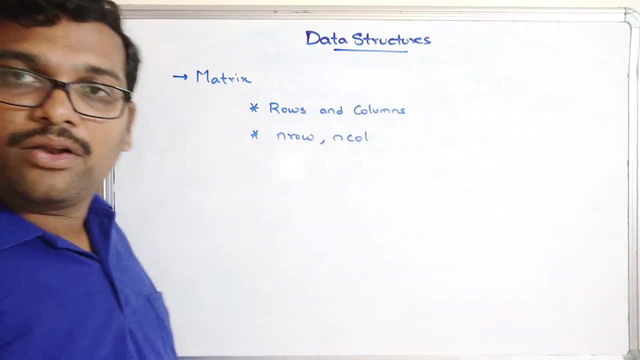 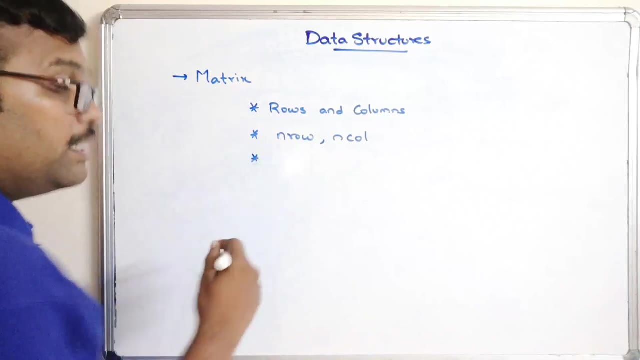 and n column n row and n column right. n row means number of rows, n column means number of columns. And also the third parameter is an optional. it is a row wise row wise right. So by default it will be the column. 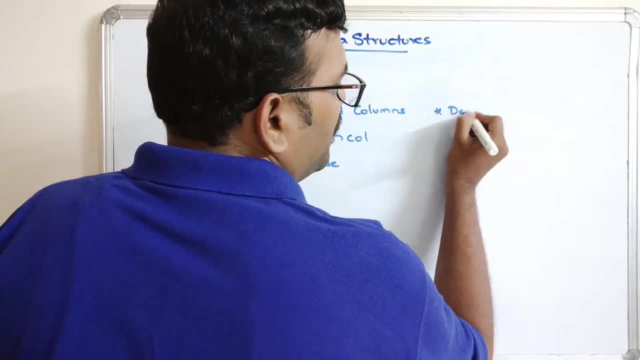 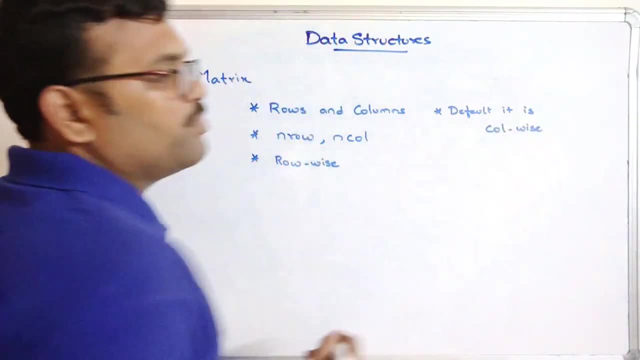 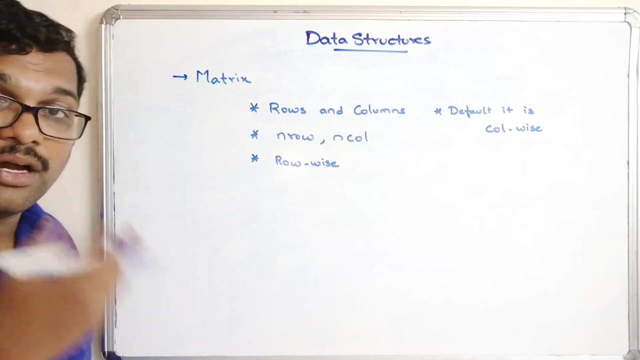 So here I will write a default. it is column wise. That means whatever the elements we are giving, that will be arranged in a column wise. So if you are using the third parameter as row wise, I mean third parameter, so we can use a row wise, we can arrange the elements. 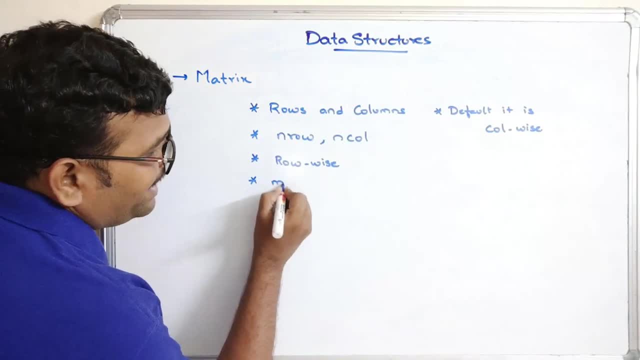 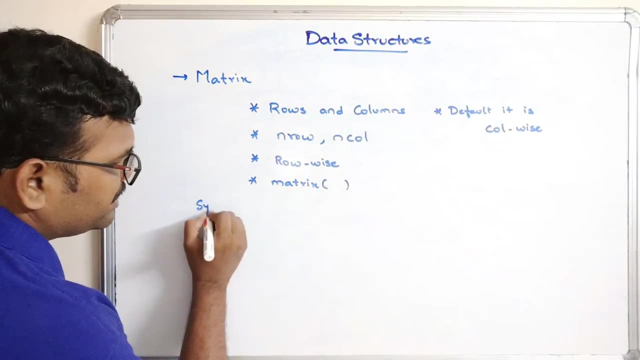 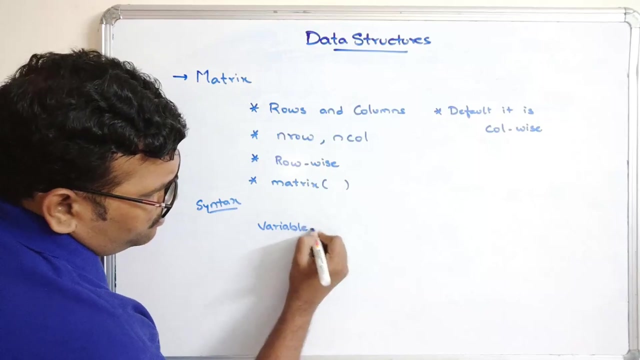 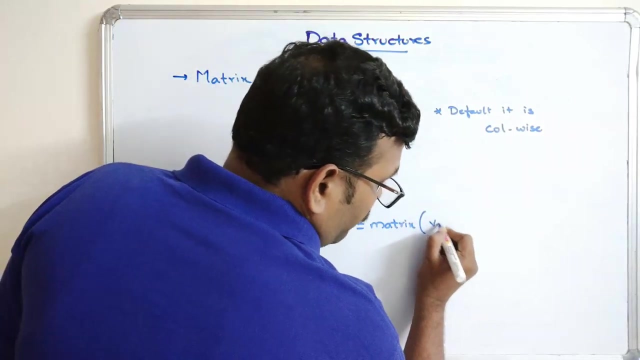 in a row, wise. So here we will use a matrix function to create a matrix, matrix function. Okay, Now I will write the syntax here. So variable name or matrix name, So we can write anything, is equal to use a matrix function. Write down the vector. So vector is nothing but a data. 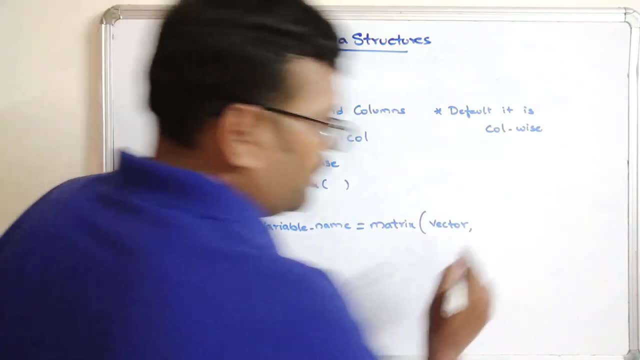 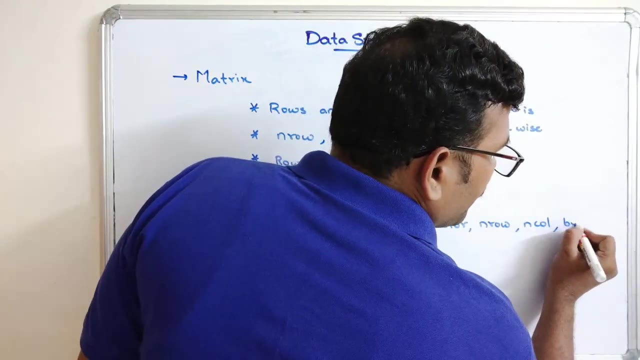 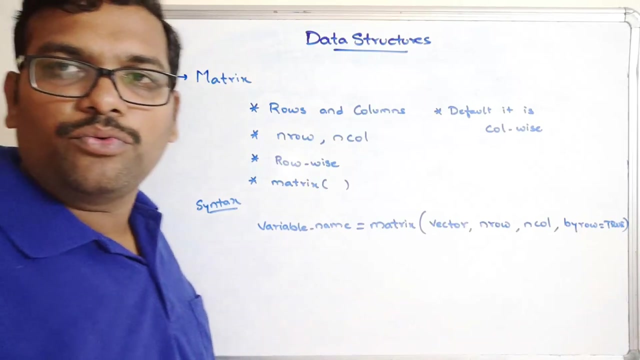 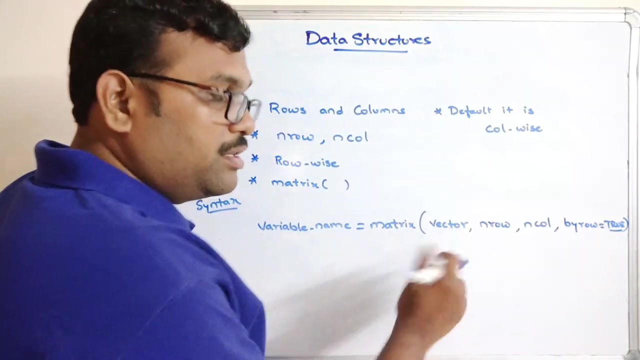 So complete data should be written as a vector here. Vector n, row n, column, and the third one: by row is equal to true. By row is equal to true. So capital letters right. Boolean data type is in capital letters, true. So this is a vector. This is a complete data Data we need to fill in a matrix. 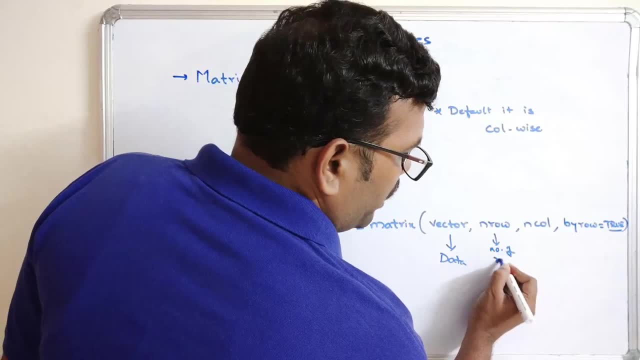 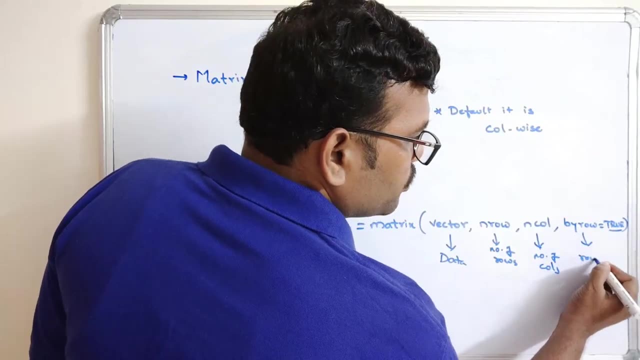 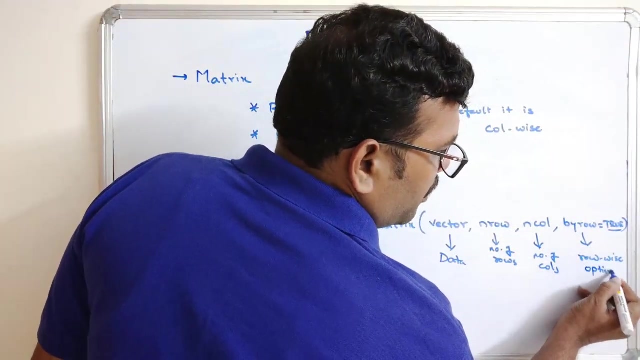 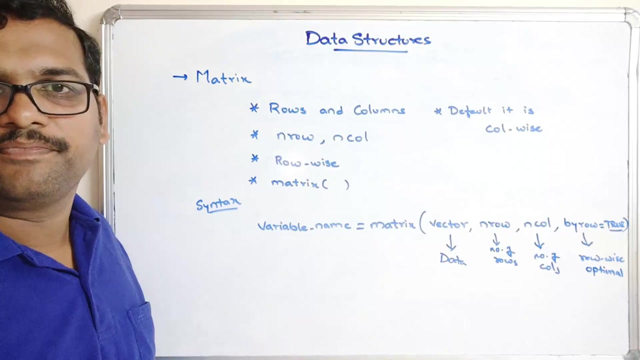 And this is a number of rows we require And this is a number of columns, And this is a row wise ordering, Row wise ordering. So this is an optional thing, This is an optional parameter. So in the absence of this by row parameter, the data will be arranged in a column bus. For example, consider a vector. 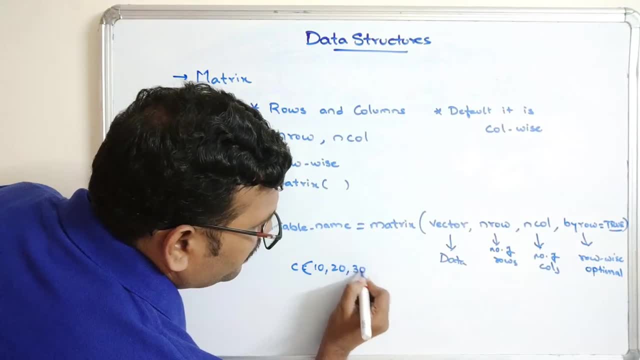 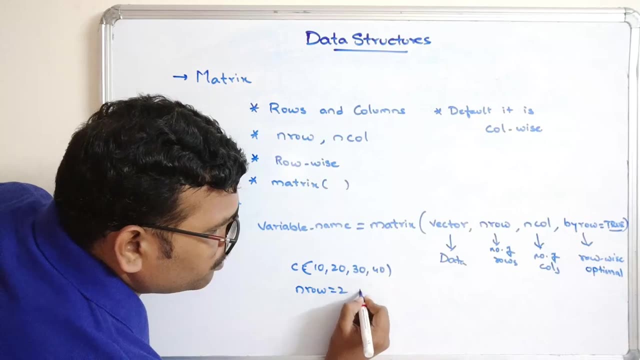 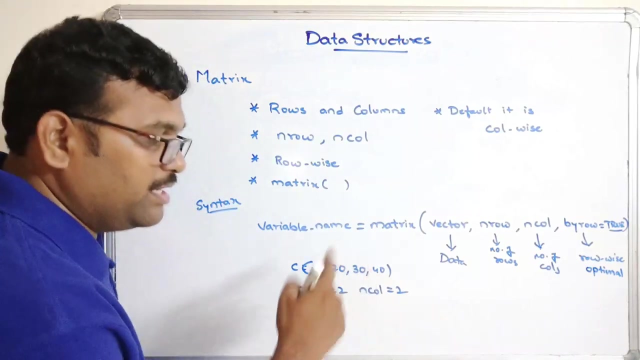 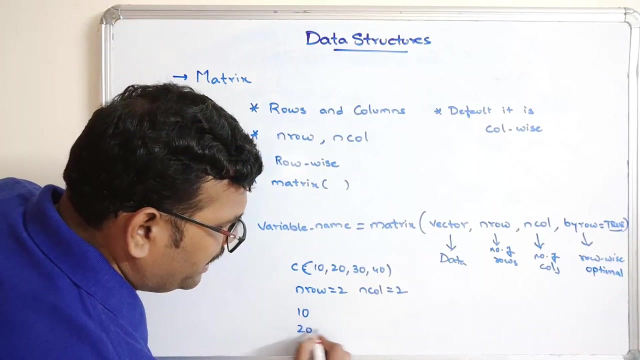 So 10,, 20,, 30 and 40. And if you want to give number of rows, n row is equal to 2, n column is equal to 2. That means 2 rows and 2 columns. So first the arrangement will be done in a column bus Right. See So 10, 20,, 30 and 40. So the arrangement will be done in this way. 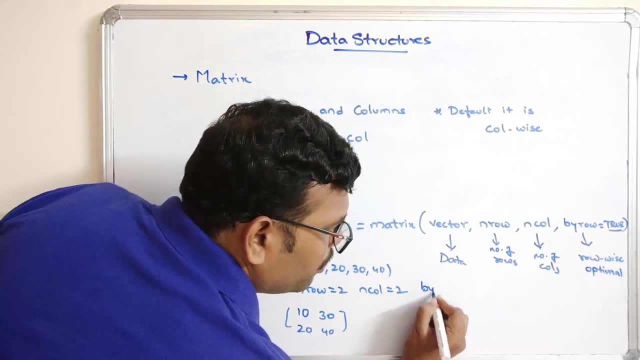 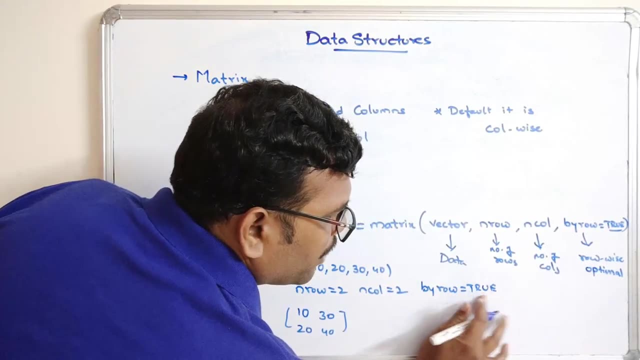 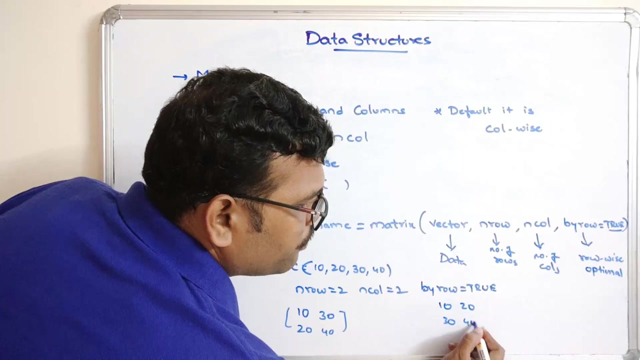 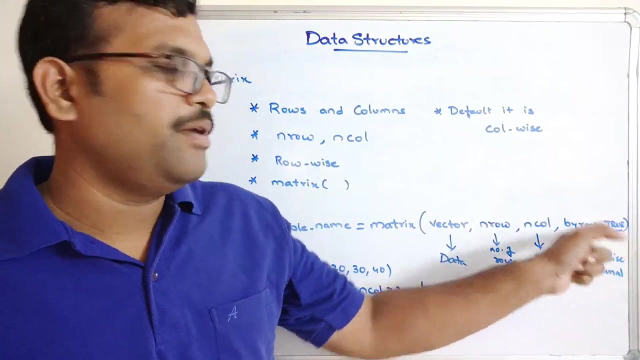 And if you add one more parameter, this by row, by row, is equal to true. Right Now, the elements will be arranged in a row: wise. Row wise means 10,, 20,, 30 and 40.. The elements will be arranged in this way, So that is the importance of the last parameter- by row. So this is an optional parameter. So, in the absence, data will be arranged in a column bus. 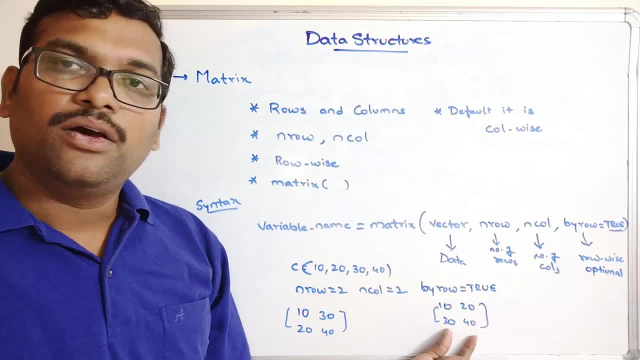 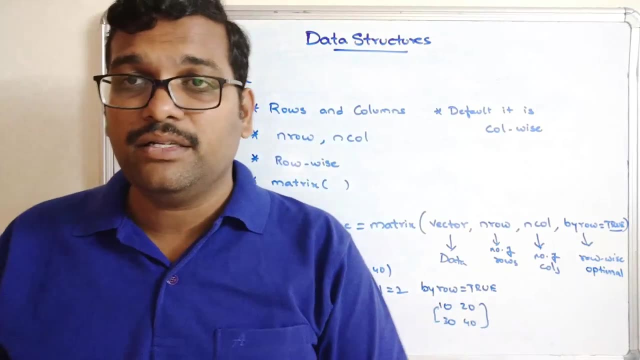 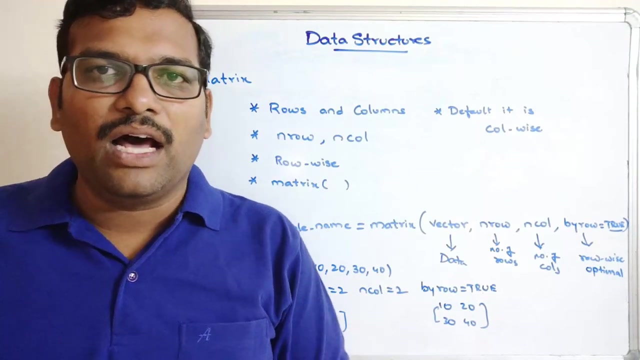 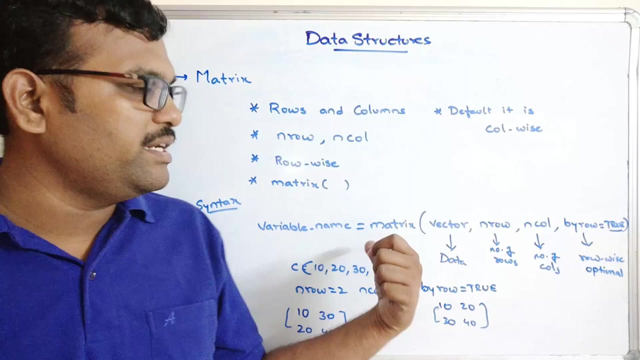 In the presence. data will be arranged in a row, wise Right. So this is all about our matrix. So we have seen a different data structures, a vector list, data frame array and a matrix. So all these are available in our R programming. Now we move on to the R studio, So I'll explain, I'll show you the implementation and the syntaxes of all these data structures. 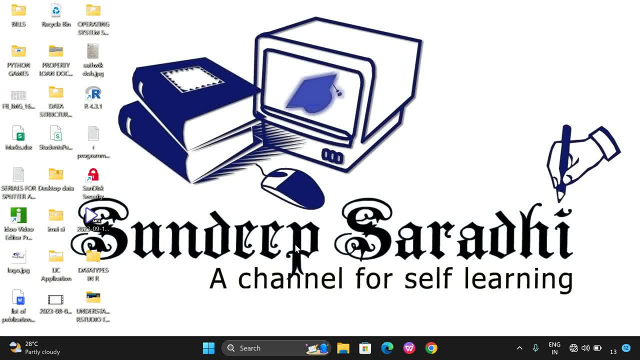 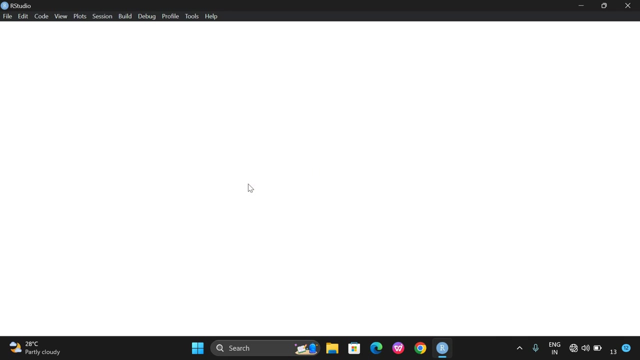 So let us move on to the system. So hello friends. So just now we have seen the theoretical part of different data structures in R programming, So we have seen the syntaxes. Now we'll see the implementation part, So how we can implement these data structures, The complete basic thing. So in depth we'll go in our further concepts. Right Now let us open the R studio environment. So once it was open, so we'll go one by one. So starting from the vector, 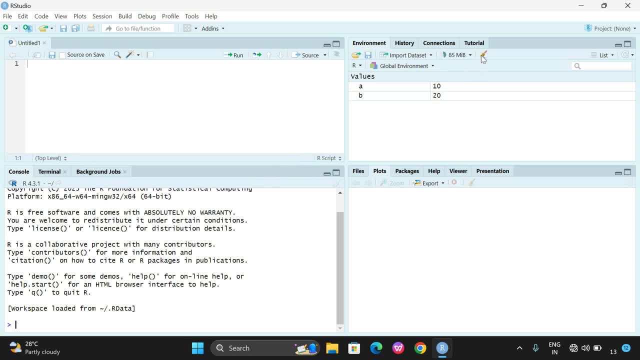 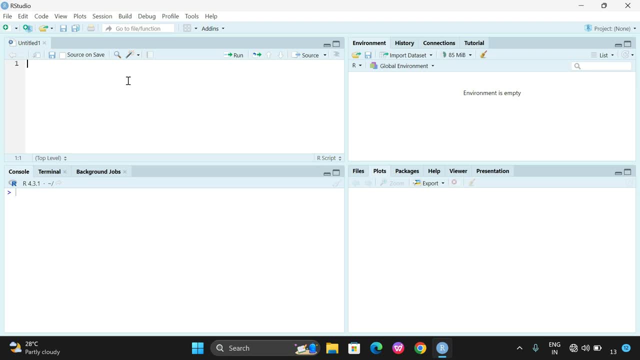 Followed by a list matrix array and a data frame, Right. So let us write a small- I mean initialize- a vector here. So some V is equal to C of. Let us give the values, So 10 comma, 20 comma, 30 comma, 40 comma, 50. And let us print that particular vector here. So execute the complete statements, So go here. 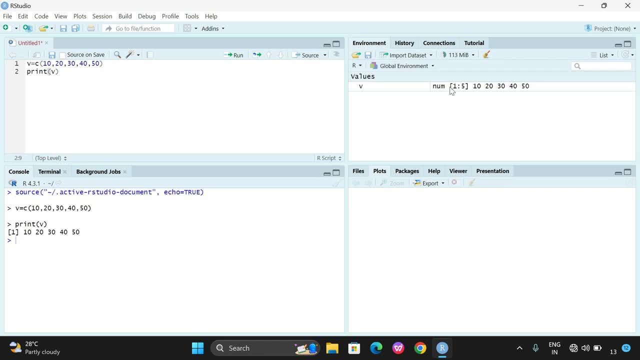 So execute. You can get the elements here Right. So this environment variable, So here indexes 1 is to 5 and the values will be printed in this particular output console. Now let us try with the different data types and execute C. It was accepted. So we have studied that a vector is a single dimensional path, So where it can accept. 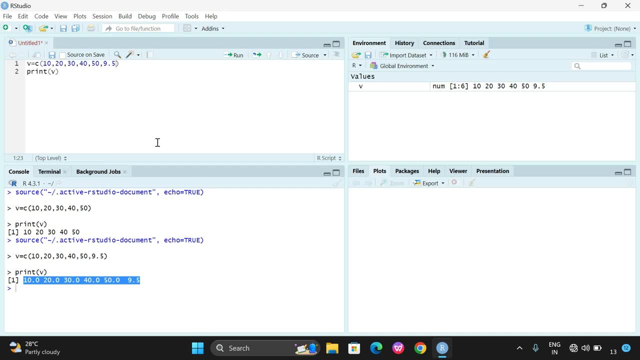 Multiple elements of the same data type or not a different data type, because you can observe here. So whenever you gave in 9.5, you can see every element have been converted into a float. So unless there is a 9.5 here, So it was executed. But all the elements are enough integers Right, So here it will accept the homogeneous elements. That means the same data. 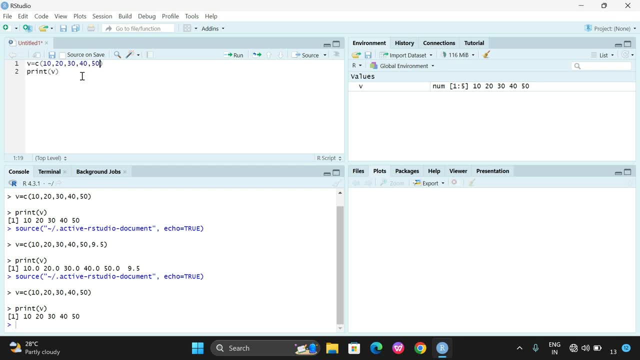 Now we'll move on to the next one. That is a list. So let us change: L is equal to. in order to create a list, We need to apply the list function. So list function and give the elements and it is nothing. but it's also a single dimension, But the elements can be of different data types. It will accept a different data types. So if you give the same thing, 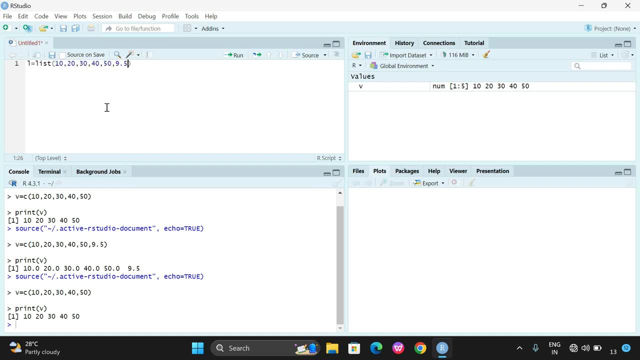 See, if you give the same elements, That means some five elements of integers and one a float, and I'll print L. and now you can observe, See, the five elements are of integer only and the last element will be the float value. So all the elements will be remained safe. That means it will accept. 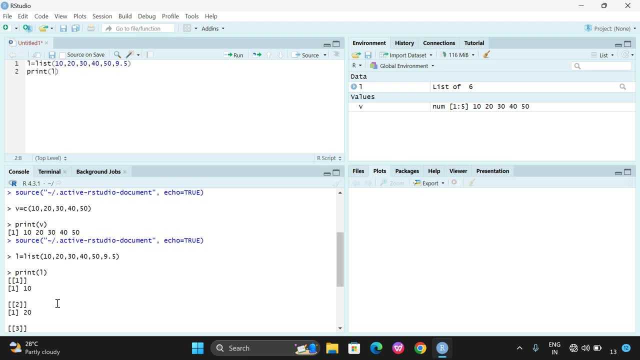 The heterogeneous data types. That means a multiple data type elements, Right, So vector is a single dimension and the list is also a single dimension. But that So the difference over a vector and a list is in a vector. it will accept only a same. 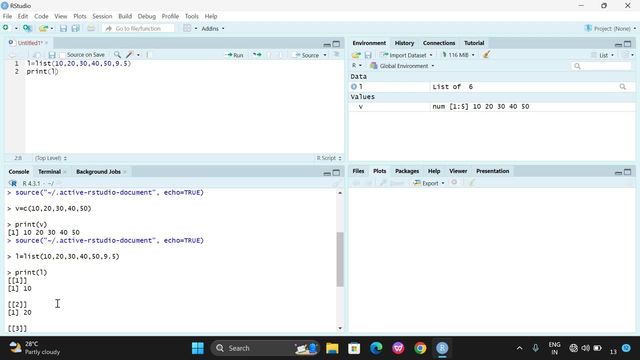 data type of elements and in a list it will accept a multiple data type of elements. right Now we will move on with the next one, that is a data frame. So let us create three vectors. So data frame is a tabular representation. just now we have seen, right. 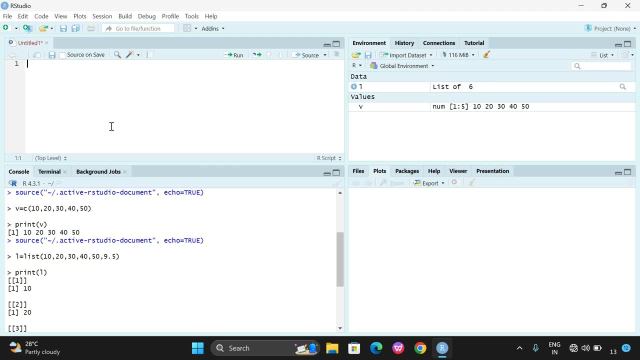 So, in order to represent any data in a tabular format, so we can go with this particular data frame and here we can give multiple vectors and we can collaborate all those vectors into a data frame so that the data will be displayed in a tabular format. 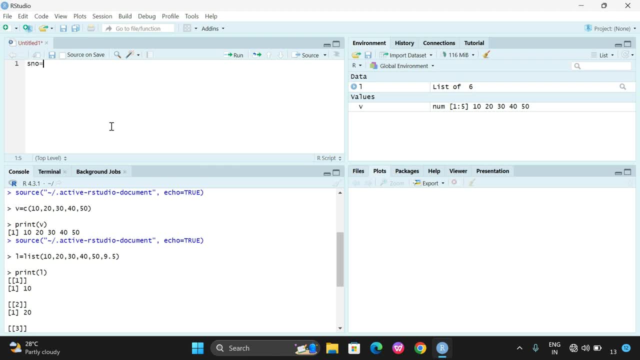 So let us take some student details. let us take some S number is equal to C of some 101,, 102,, 103.. And so these are vectors. right, these are vectors. So student name is equal to C of you can give A, B, C, D, E, F, G, H, I, V. 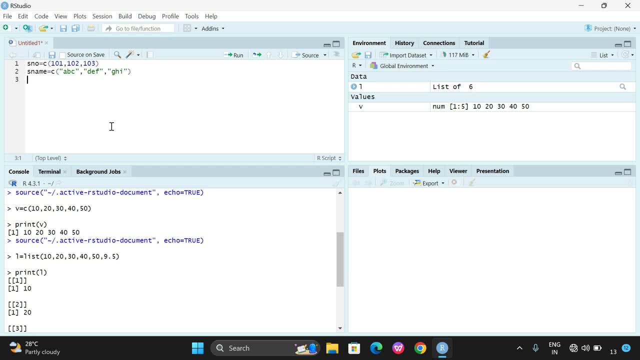 So all are of same data type, because this is a vector and it will accept only the homogeneous data. that means every element should be of same data type And I will go with the percentage. student percentage is equal to C of. let us give some. 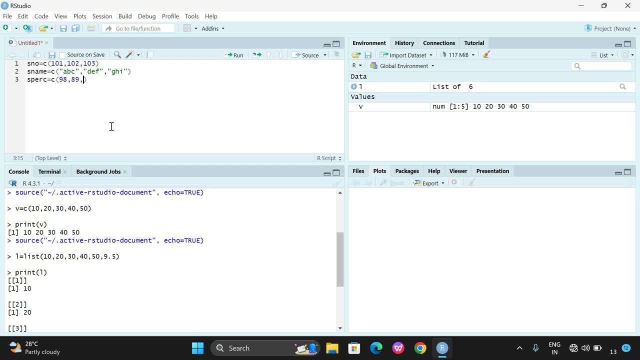 98. Now we will combine all these vectors in a data frame, So the complete data will be available in a tabular format. let us take So D, F is equal to the function, is data dot frame and you can pass all these things S. 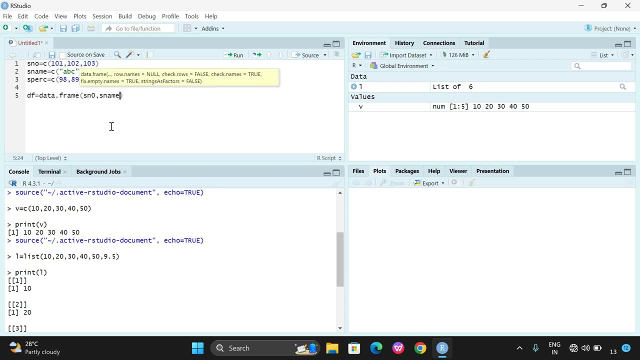 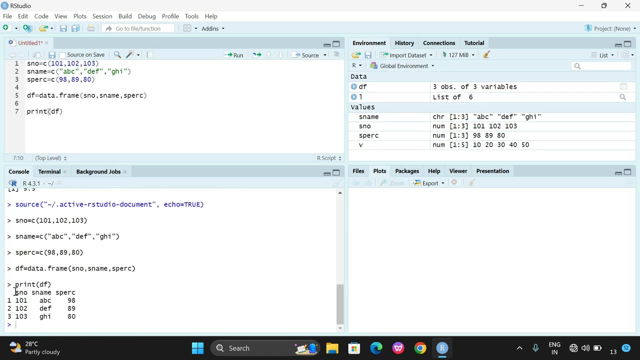 number, S name, sorry, S number N O, I think we have given so- S name and S percentage. Okay, Now you can just print a data from D F. So if you execute here, you can see S number, S name and S percentage and you got the complete. 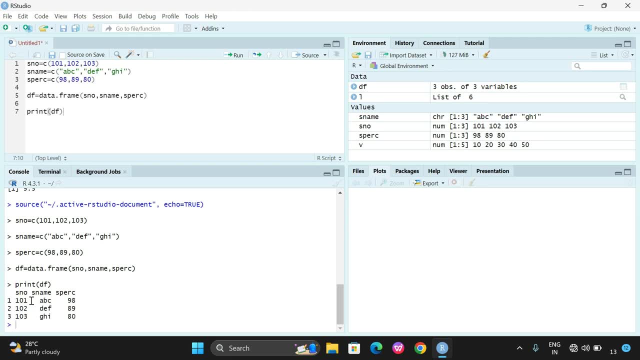 details in a tabular format. So 101 is a serial number and a serial student name. student number is 101, student name ABC and student percentage 98. So here we have given an individual vectors But We are seeing the tabular format. 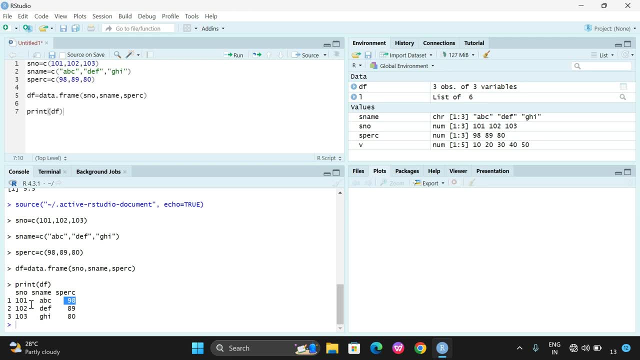 So, in order to represent any data in a tabular format, we can go with the data frame right, And the next one is an array. So we know that array is also a homogeneous elements. Okay, So here we use an array function to create an array. 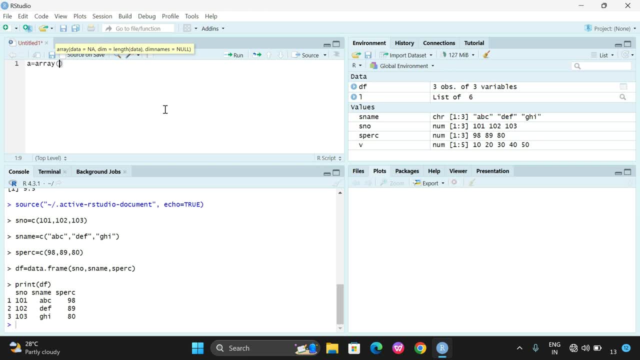 So A is equal to array of. So give a vector. give a vector C of- I'll use some 10, 20,, 30,, 40,, 50, 60. And in array we need to specify the dimensions. 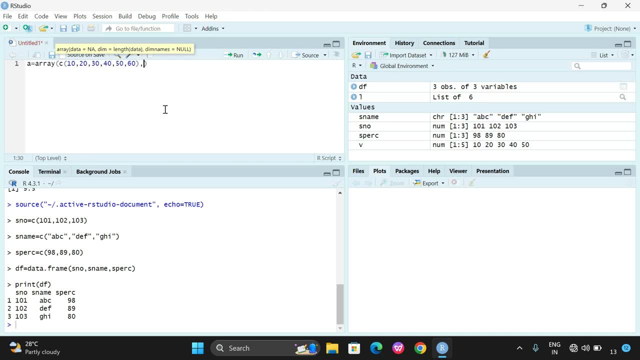 So array can be of N dimensions, right? So it will be having a two by two array, two by three array. So dimensions means two by two, that means two rows and two columns. We call them as a dimensions, right? So here we need to give a second parameter. 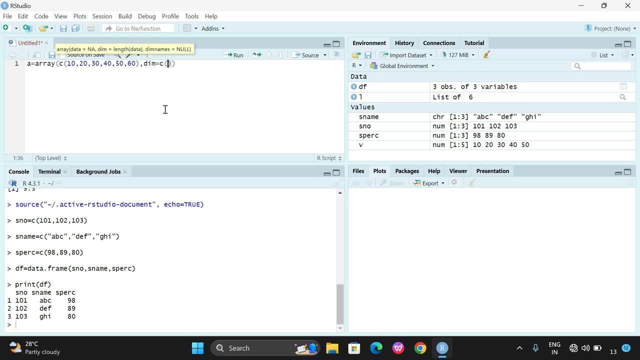 D, I, M and give the dimensions as a vector, as a vector, So in the dimensions, three parameters: the first one represents the rows, second one represents the columns and the third one represents number of arrays of the total dimensions. So here we have given some six elements. 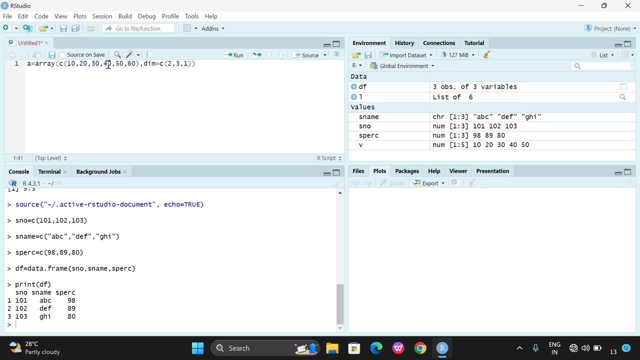 I'll use some two comma three and one, So that implies the dimension is two by three. matrix. The order of a mat. Sorry, The array Is it? It's a two by three array of one array. right, It will be having only one array, and now we can see print A and execute. 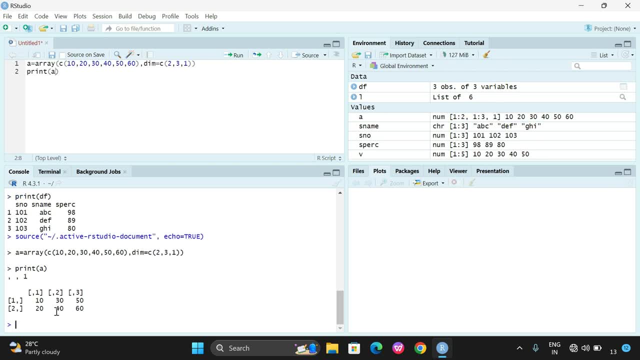 So you'll be getting the same thing: see 10,, 20,, 30,, 40,, 50, 60.. So everything will be in a column model, right? So you can observe the two rows and the three columns- two rows and three columns- and the. 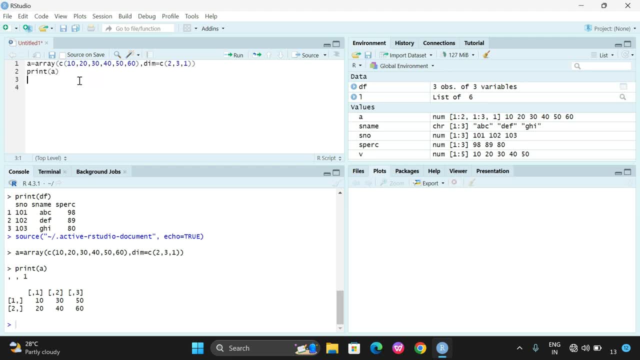 same thing. We can give a matrix, We can, We can, We can give a matrix. So M is equal to. we need to give the matrix function. So in the matrix again you need to take the complete values, So C of 10,, 20,, 30,, 40,, 50,, 60, and here we need to give the number of rows and number. 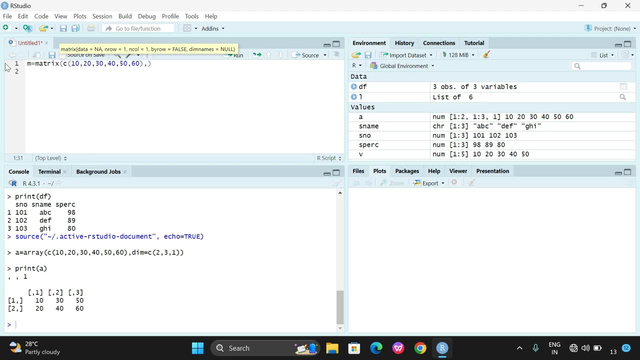 of columns, So order of a matrix. right, So M row is equal to: I'll give you three rows, And Okay. Okay, So M column is equal to I'll give it two columns, right, And simply print M and you can observe here. see the three rows and the two columns. 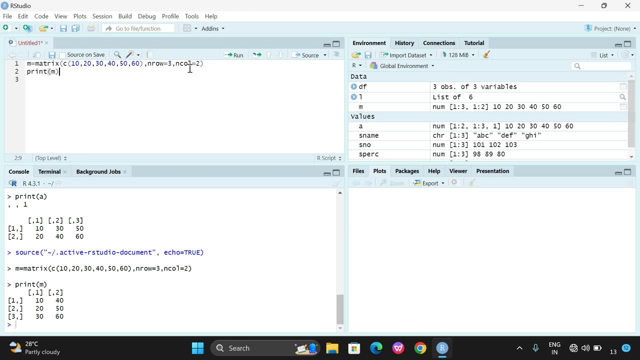 So if it is an array, we need to specify the dimension. So here there also, we need to specify the number of rows and columns, but we call it as a dimension and come into the matrix. Here we need to give some N rows and N columns and you can observe, by default it will be. 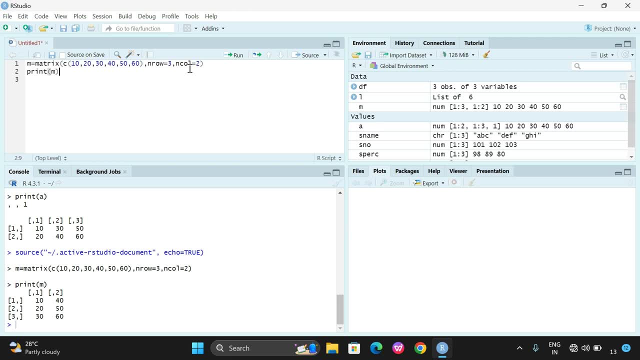 taking the elements as a column wise. If you want to arrange them in a row wise, So you need to add one more parameter called by row is equal to true, So elements will be arranged in a row wise. So you can observe here: 10,, 20,, 30,, 40,, 50,, 60.. 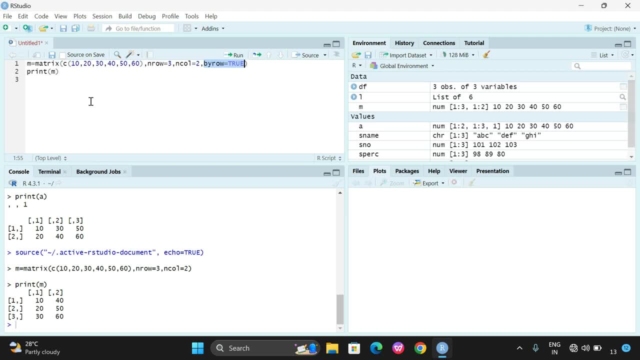 So if you are not giving this by row parameter, So the data was Filled with a column, wise, see 10,. 20 is in second, second column- I mean first column- and 30 will also be in the first column. 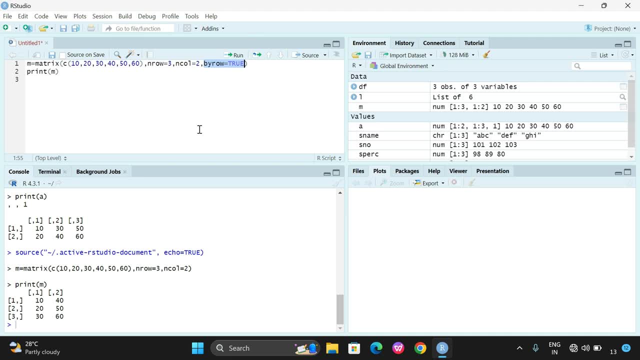 Then only 40, 50, 60 will be arranged in second column. Now, if you add this parameter by row is equal to true And if you execute, you can observe 10 and 20 will be the first row, 30 and 40 will be. 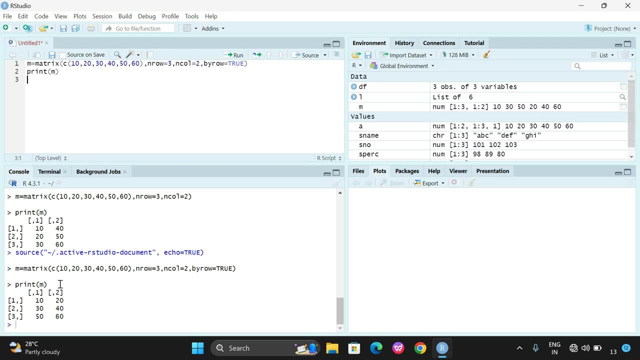 the second row and 50, 60 would be the another row. So that means the elements will be arranged in a row order. Okay, So we'll change the data type, So 30.4, 40.5, and still execute the same thing. 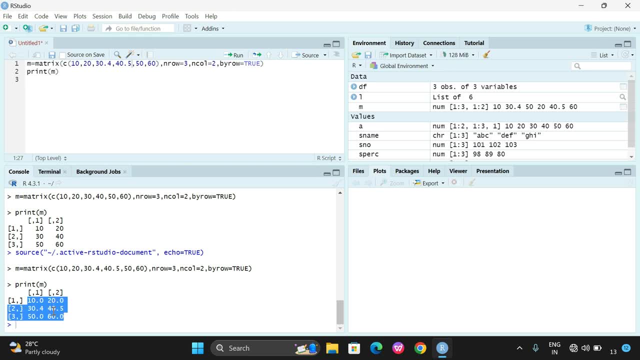 And you can observe, this is a homogenous. Everything has been changed to float, Everything has been changed to flow right. So a slight difference among the vector and a list, as well as an array and a matrix, right. So hope you understood.